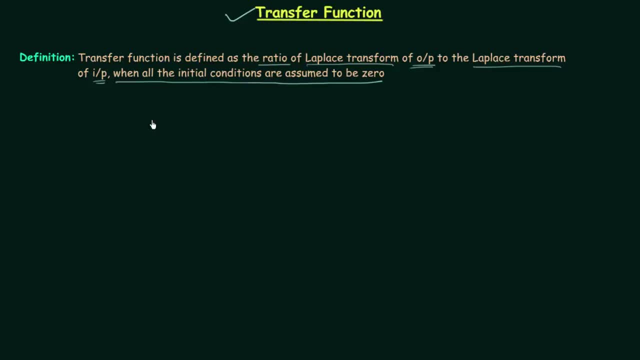 is very, very important. Without this point, you cannot define the transfer function. I will explain the significance of this point after some time, but first we will write down our transfer function. The transfer function is represented by HS. It is a complex function. The transfer function is a complex function and the variable S is also complex. The variable S is also complex. 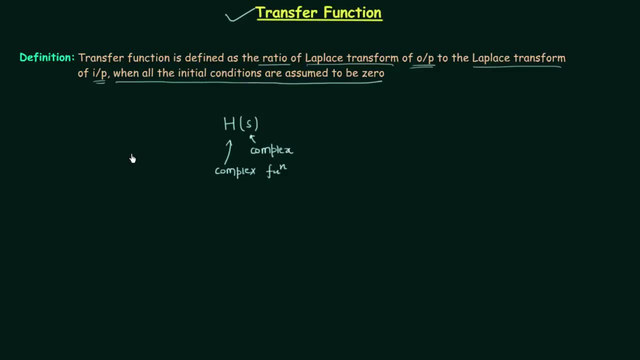 And the transfer function is easily obtained after taking the Laplace transform of impulse response. HT is the impulse response and after taking the Laplace transform of impulse response, you will have the transfer function of the LTI system. And when you take the inverse Laplace transform of the transfer function, you will have the impulse response. Now, from the definition, we can clearly see that the transfer function is obtained after taking the Laplace transform of impulse response. 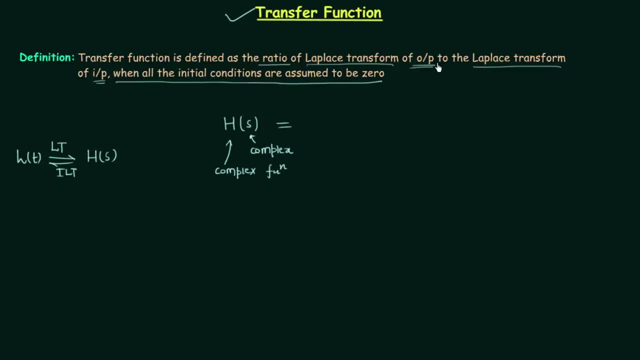 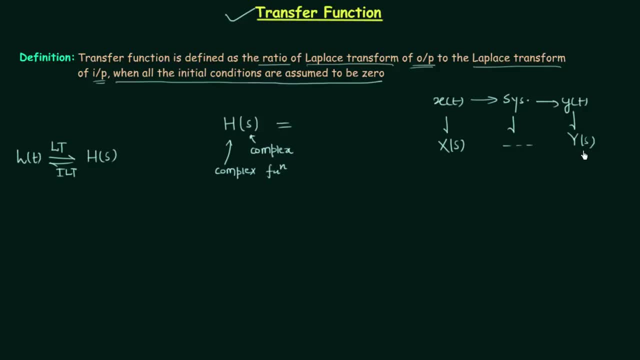 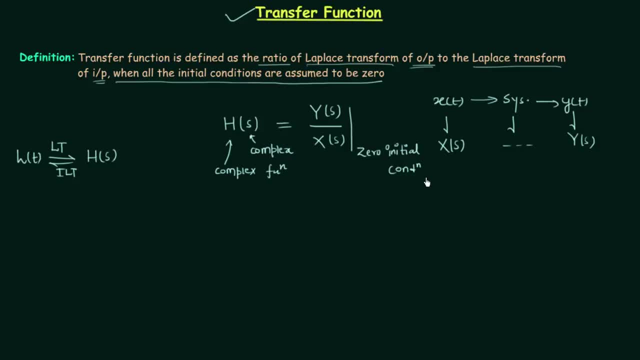 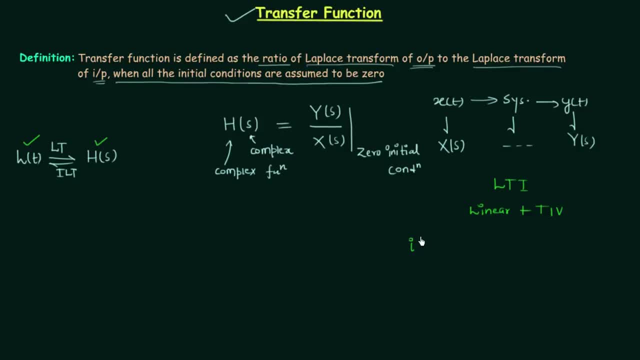 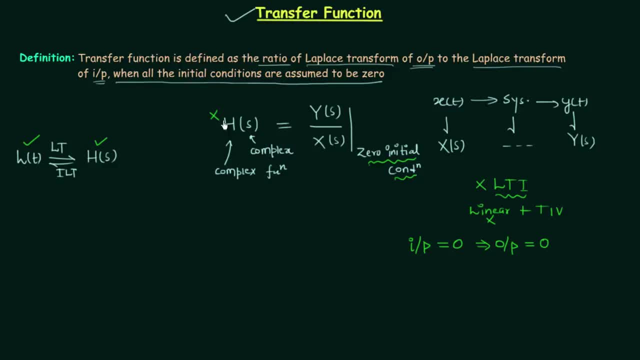 systems, we cannot define the transfer function. I will explain how the property is violated. if we don't consider zero initial conditions, The output here is the total output, the total output of the system, and it is equal to zero input response plus zero state response. I will write. 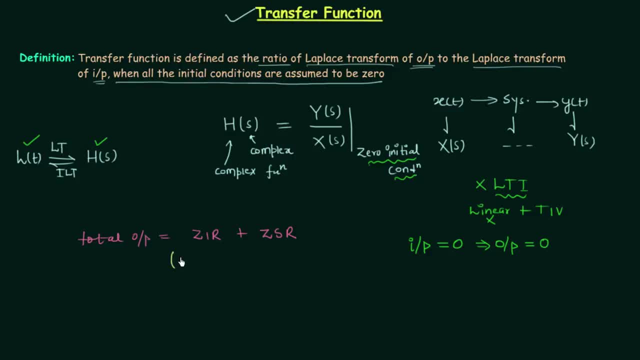 down the names here: ZIr stands for zero input response And Zsr stands for zero state response. The first response- zero input response- is when the input is equal to zero and the response is due to the initial interval: zero status. youibe its기� Rück blev 인, 즉 인 intentar 모은 정당에. 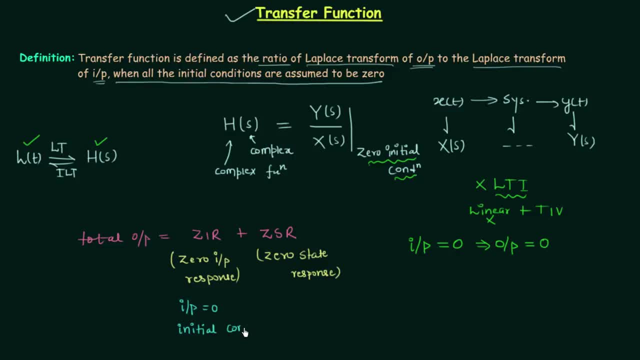 conditions, initial conditions due to initial conditions and zero state. response is the response when the input is applied. response means the output and because of these two responses we have our total output. now, if you don't consider the initial conditions to be zero, then you will have Z IR. Z IR will not be equal to 0 because the initial conditions are not equal to 0. the 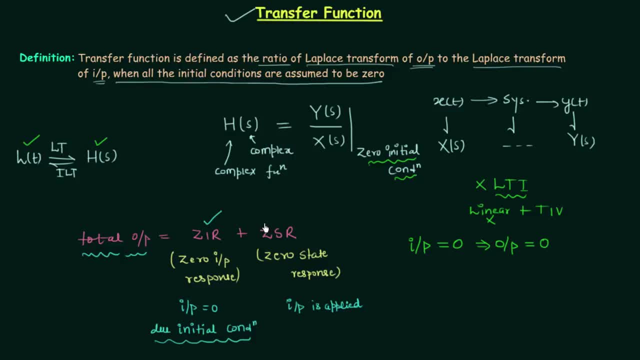 input is equal to 0 in this case, now consider the input equal to 0. the input equal to 0, Z SR will become 0, so no Z SR, but the total output will not become 0, even when the input is equal to 0. now listen to this once more: the total output is equal to Z IR plus Z SR. 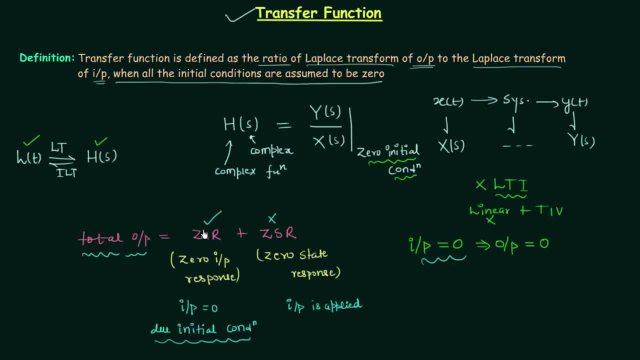 Z IR is the zero input response. it is the output of the system due to initial conditions. we are not considering the initial conditions to be 0, so Z IR will not be equal to 0, will not be equal to 0. there will be some Z IR because the initial conditions are not equal to 0 and for Z IR the 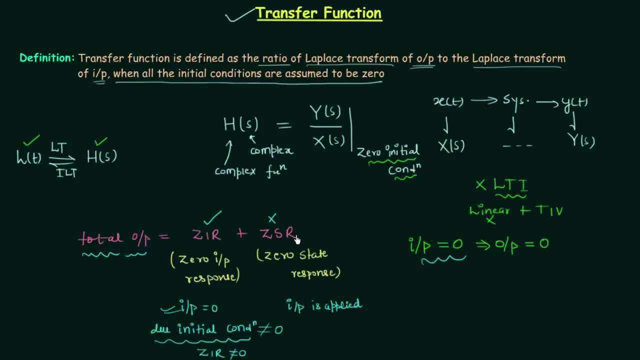 input is always equal to 0. the second output is Z SR. it is the zero state response and it is the possible input, which is 0, the zero state response. and there, if we can substitute that, then Z IR would be able to be equal to 0 and we can show return zero state response as well. 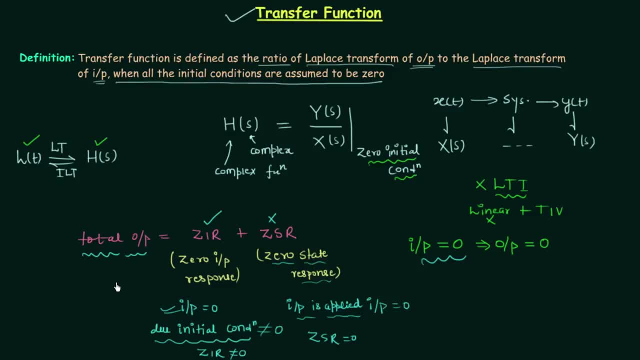 so we can write the operating empez pans on zero. the result: this input is zero and as we are considering input to be zero, ZSR will be equal to zero. ZSR will be equal to zero as the input is equal to zero. so the total output is not equal to zero. the input is zero, but the total output is not equal to zero because ZIR is not equal. 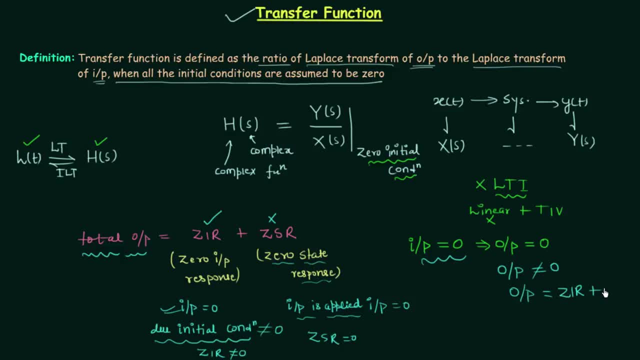 output is equal to ZIR plus ZSR. ZSR is equal to 0, but ZIR is not equal to 0 because the initial conditions, the initial conditions, are not equal to 0 and as the input is 0 and output is not equal to 0, the system is nonlinear and